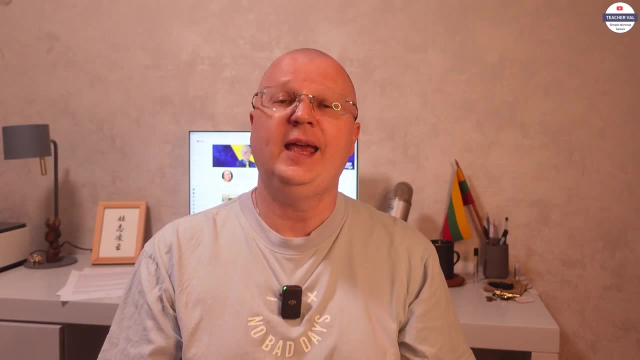 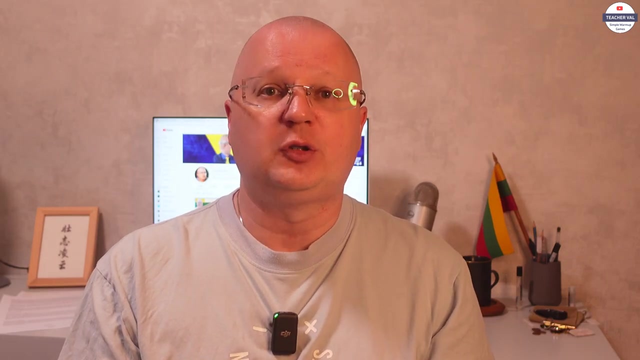 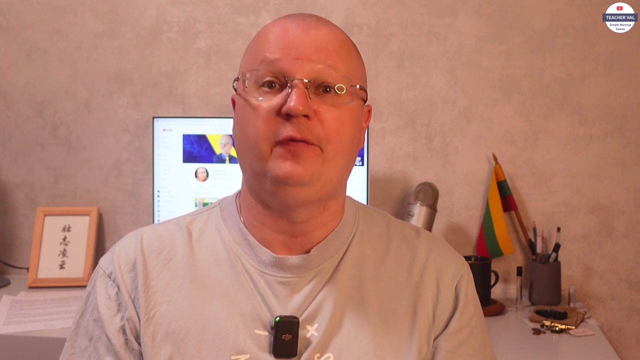 Hello everyone, my name is Val and welcome back to my channel. In today's video, I'll share three simple ESL games designed specifically for primary school students. These games require zero preparation, minimal resources and yet promise maximum fun and learning. All you need is a blackboard, a piece of 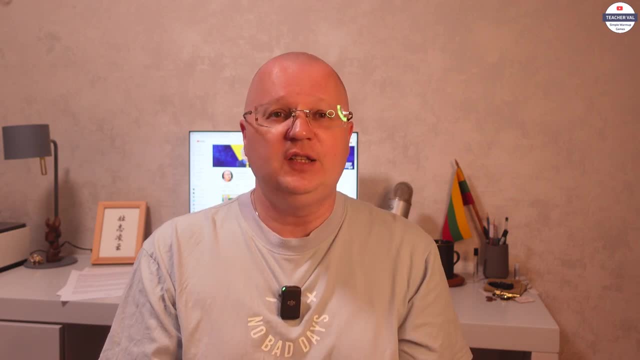 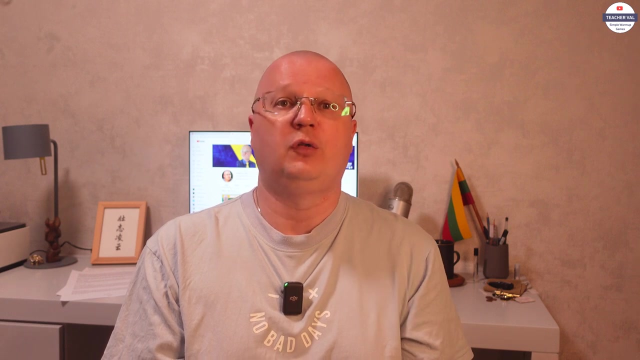 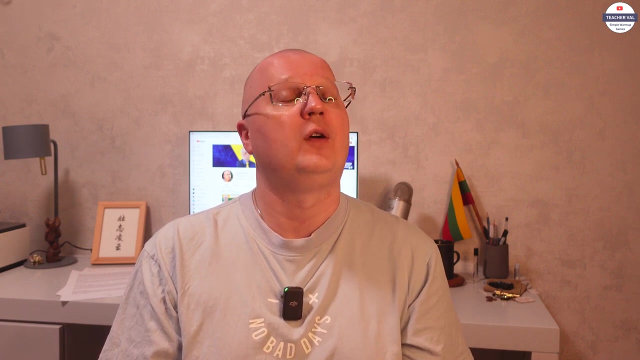 chalk and your students. These games are perfect to kick-start your class, setting a positive and engaging tone right from the get-go. They not only warm up the students, but also foster a friendly classroom atmosphere, making language learning a delightful experience for everyone. So if you are an ESL teacher, 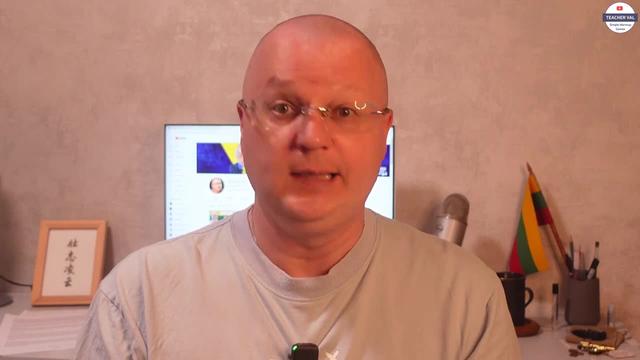 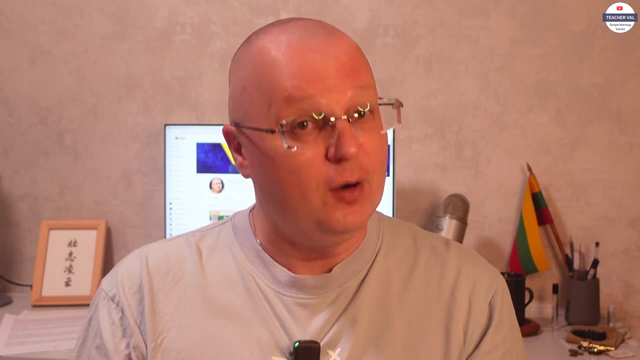 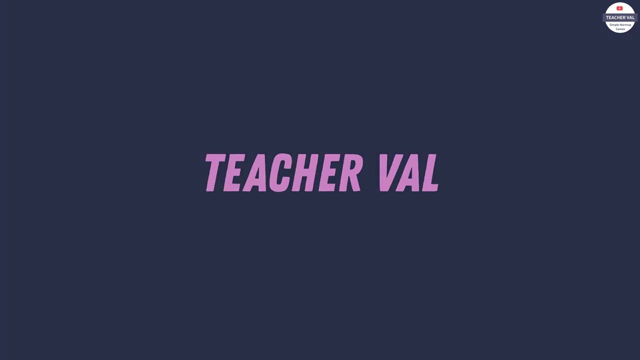 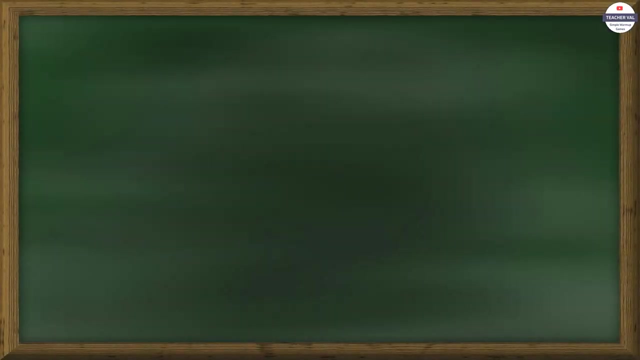 looking to bring a fresh wave of excitement into your classroom. stay tuned as I walk you through these simple yet very effective warm-up activities. Game number one: biting your tail. Split your class into two teams. Choose a topic, for example school. 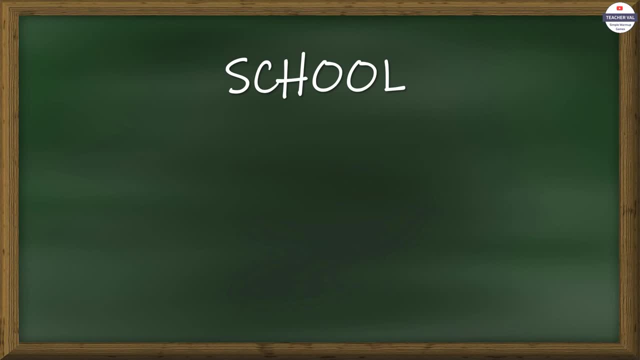 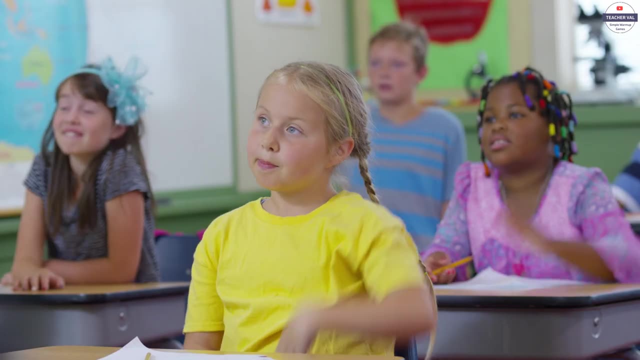 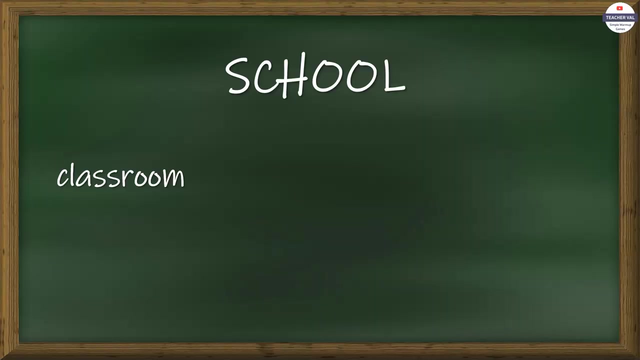 Start the game by writing a word from this category on the blackboard, For example: classroom Students from both teams raise their hands. Pick a student from one team to write a word that starts with the last letter of the previous word. Then the student from the other team does the same The game. 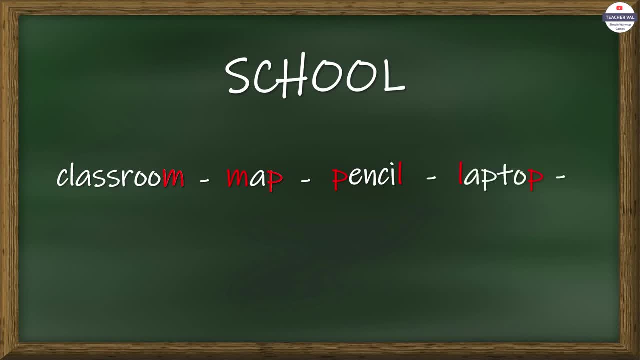 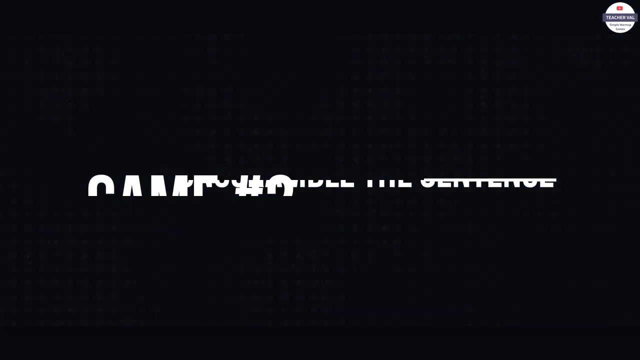 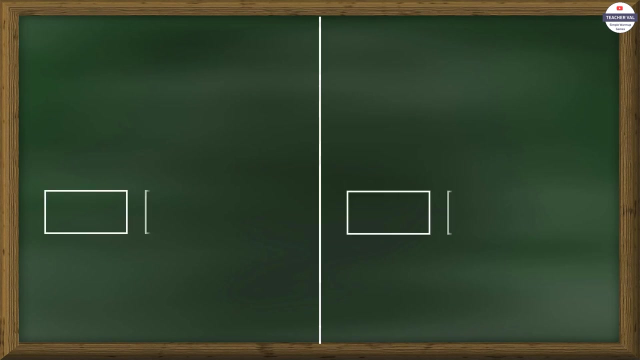 continues until next time. Thank you, No one can come up with a new word. The game restarts with a new word or category. Game number two: unscramble the sentence. Draw a line in the middle of the board to divide it in half. Draw a few rectangles on each side of the board. Write a word in. 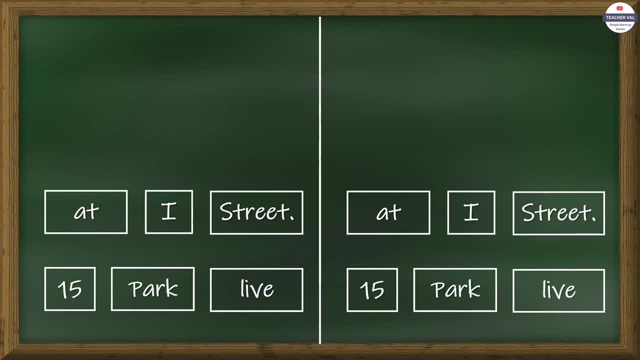 each rectangle, For example, at I street 15, park live. Split your class into two teams. Invite a student from each team to come to the board. Ask them to put the rectangles in the correct order so they make up a sentence. For example, I live at 15 Park Street. You can also ask: 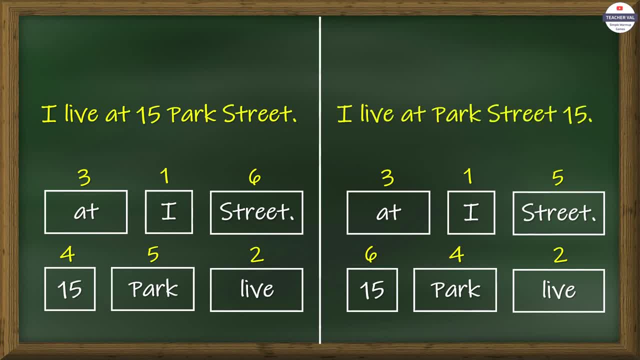 them to write a sentence on the board. Whoever does it first gets a point for their team. It's also a good way to check punctuation marks. You can remind your students that we start a sentence with a capital letter and end it with a period. 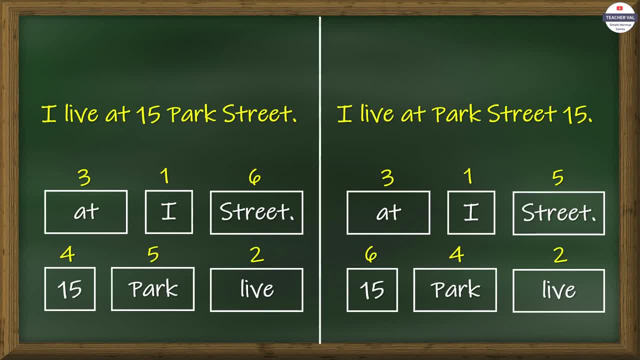 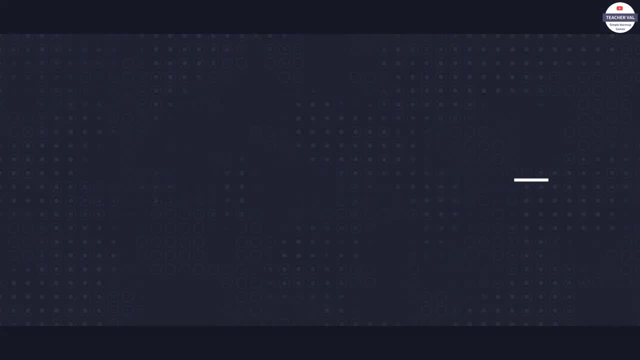 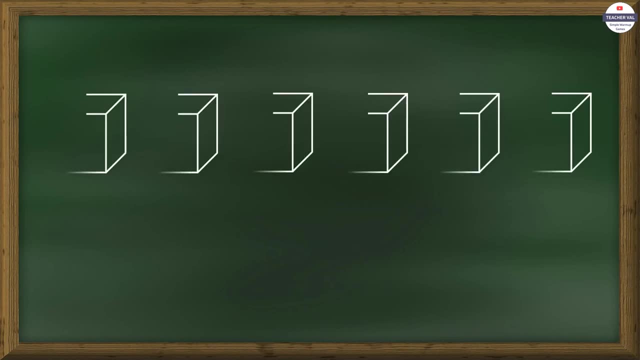 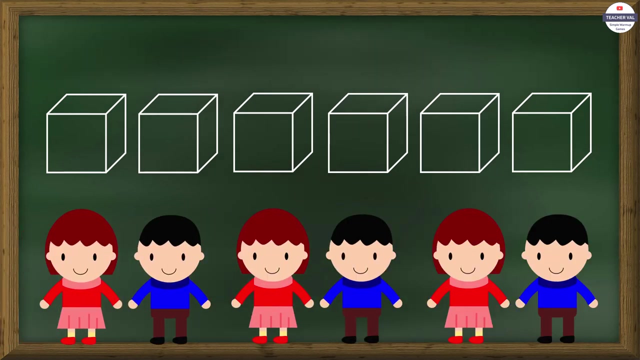 Repeat this procedure a few more times with different students. Game number three: preposition squares. play this warm-up game as a whole class activity. draw up to six 3d boxes on the board. invite six volunteers to stand at each box with a piece of. 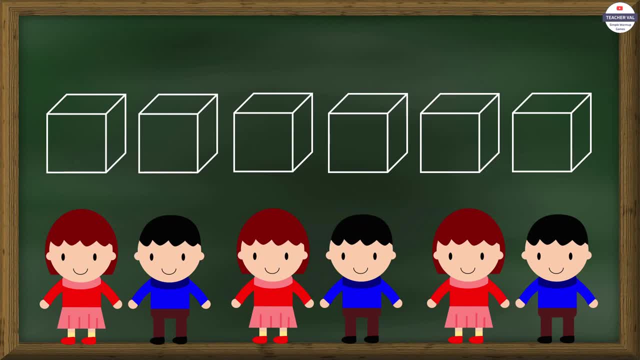 chalk, say a sentence with a preposition. for example, there is a pencil in my pencil box. your students must draw a star or any other object in the correct position on the box, as you call it out. demonstrate the correct position first when playing the game for the first time, to illustrate where to draw the stars. 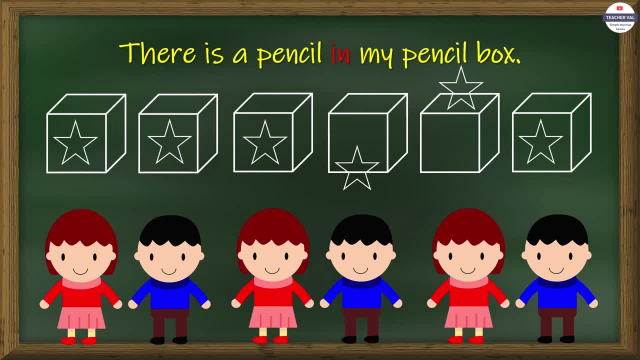 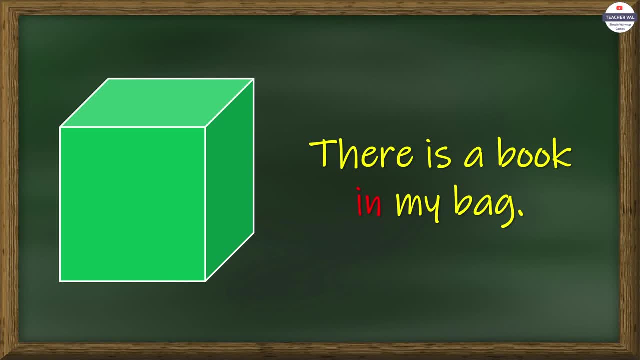 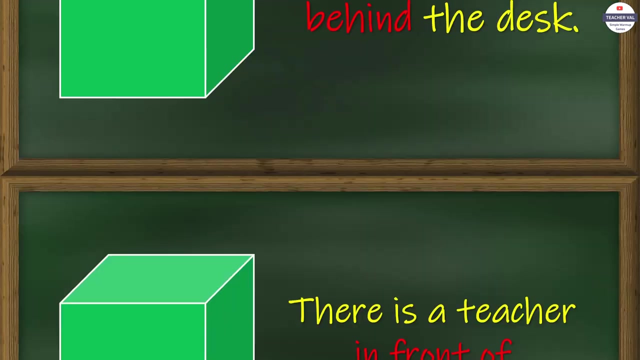 especially for the prepositions in front of and behind on a flat board. let me give you an example: there is a book in my bag, there is a ruler under my chair, there is an apple on my lunch box, there is a boy behind the desk. there is a teacher in front of the blackboard.